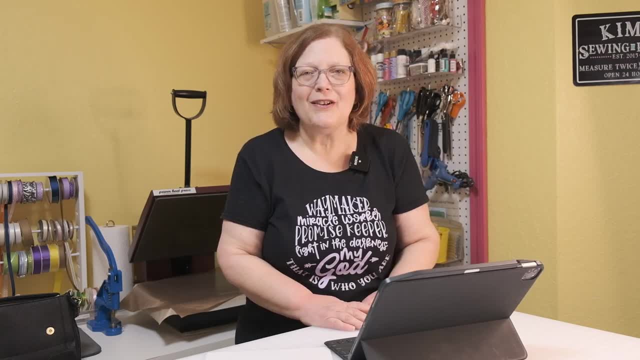 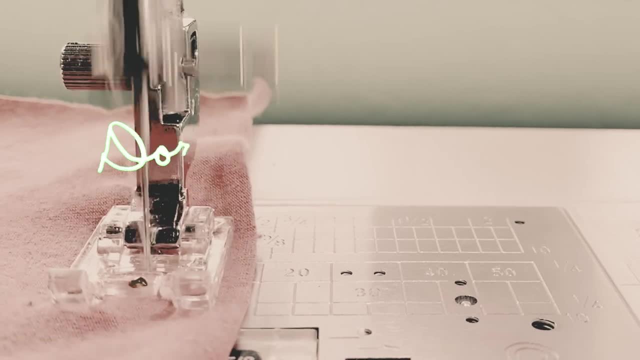 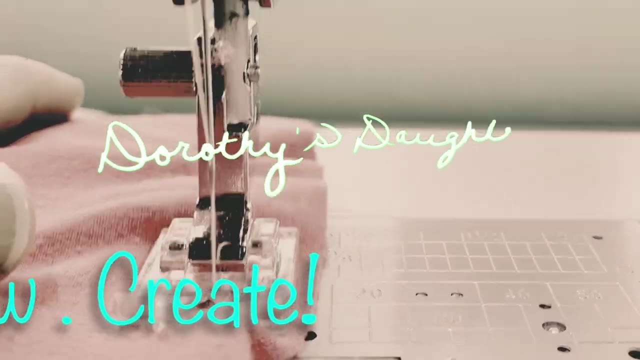 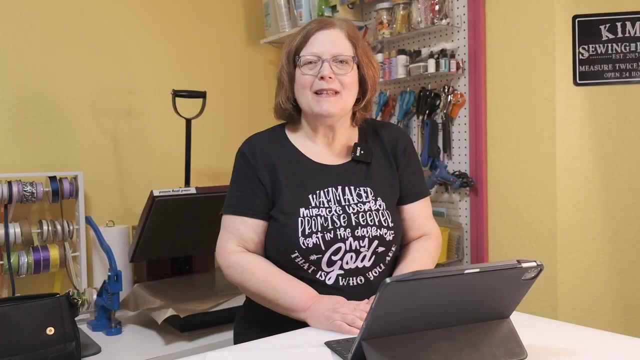 Hi all, this is Kim from Dorothy's Daughter. Welcome to my channel. Today, we're going to talk about the top 10 free patterns for kids, So stay tuned. Hi, this is Kim from Dorothy's Daughter. Thank you so much for being here with me today. 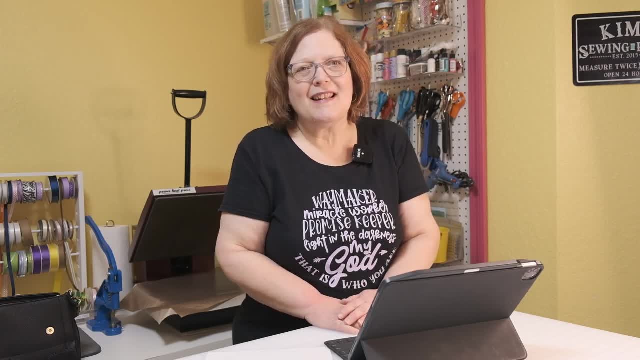 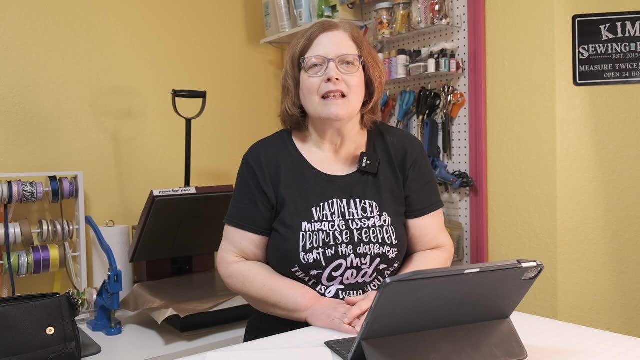 This is the place to be if you want to take your sewing to the next level. So a lot of emphasis is put on saving money while you sew, and I'm all for that, because we all need to just save money wherever we can. So today I thought I'd share with you. 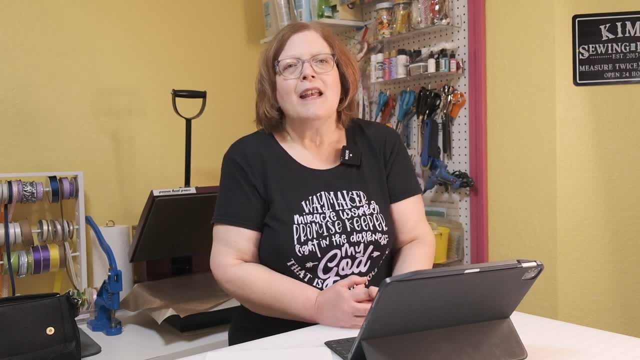 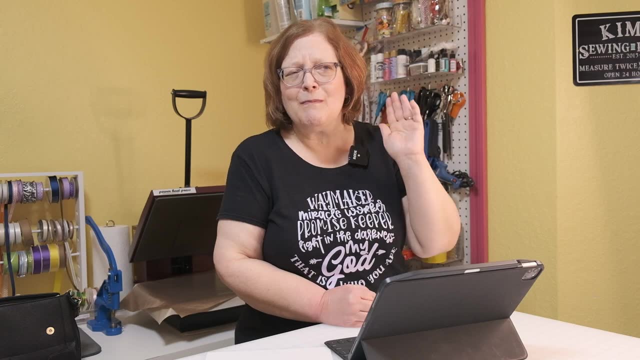 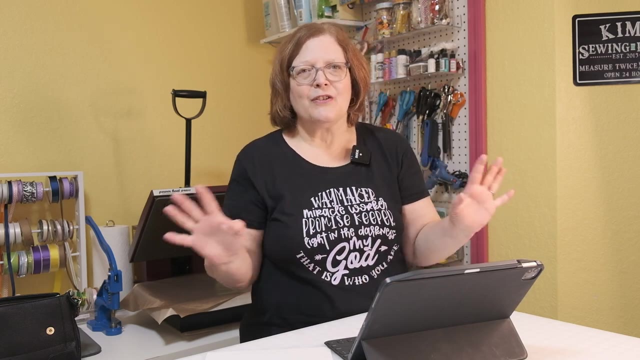 my favorite kids patterns online that happen to be free. So, rather than being 10 patterns, these are going to be 10 different designers who, some of them, happen to offer more than one free pattern. So a little bit more than 10 free ones, but there should be a lot to pick. 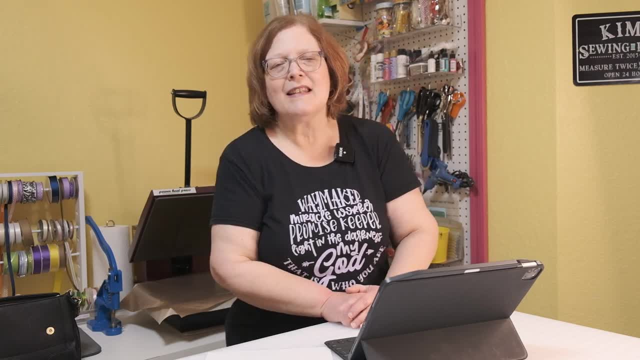 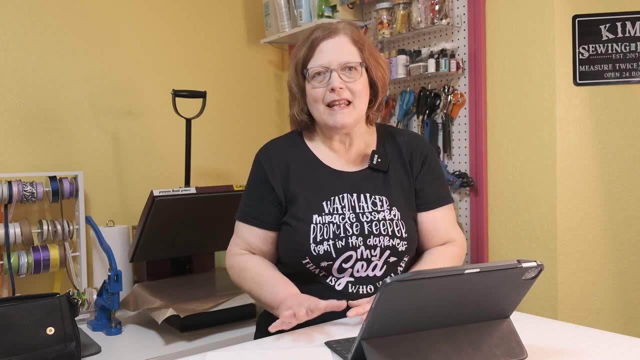 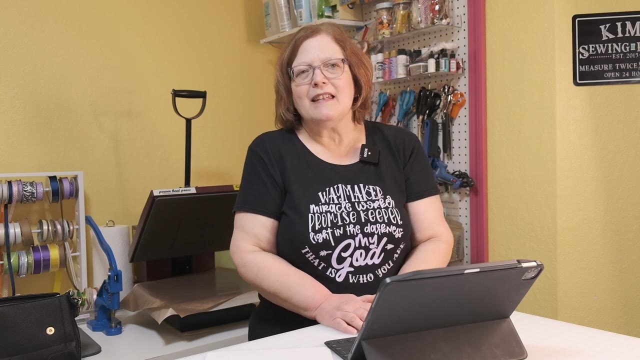 from for you, if you sew for your grandkids or your kids. This is the time of year when everybody needs play clothes, So try to really keep them to be like basic staple things for you. And we will get on with that in just a moment. But first of all I just want to remind you that, if you'd like, 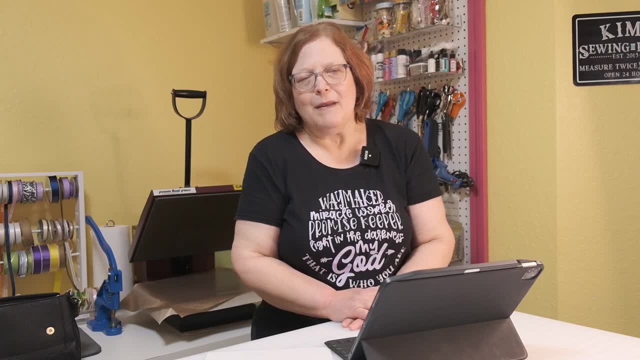 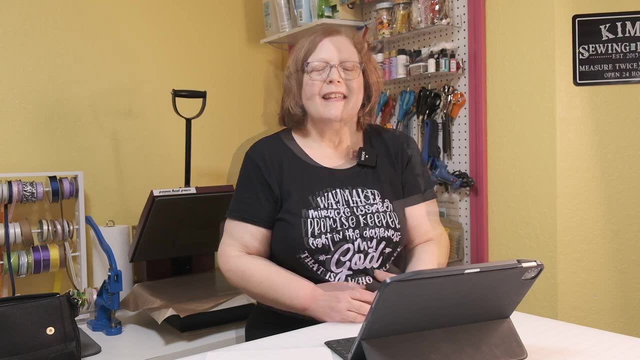 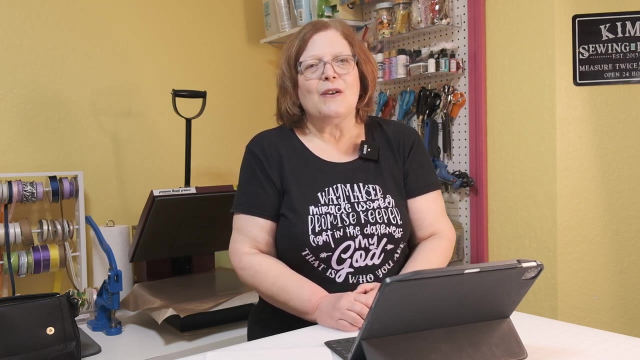 to help this channel. the very best thing you could do is subscribe and then like or share the videos, just so that YouTube puts them out there as suggestions for people more often. So we're at 15,000 subscribers, which blows my mind completely, in two short years. So I'd love to 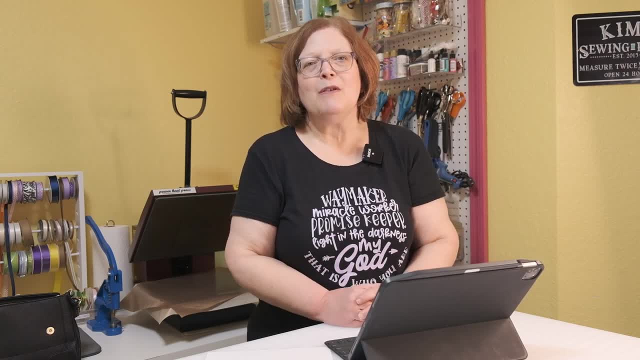 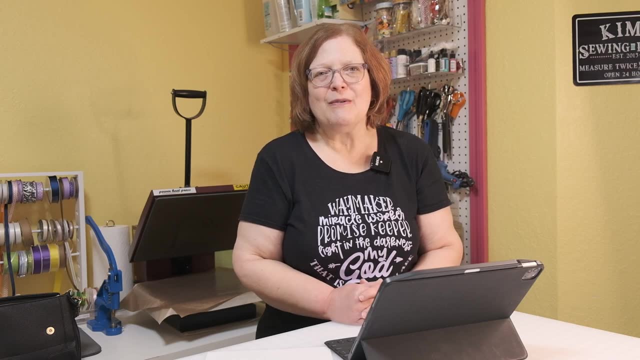 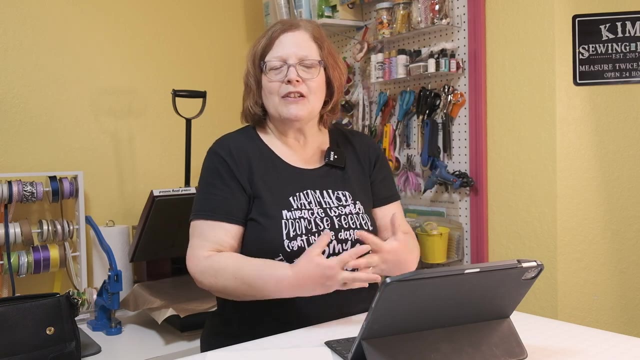 have you come along and be part of the community that is known as Dorothy's Daughter. So hit that subscribe button, like and share the videos that you would love to share with other people, and join our Facebook group and get in on the fun. The first designer I'm going to talk about is 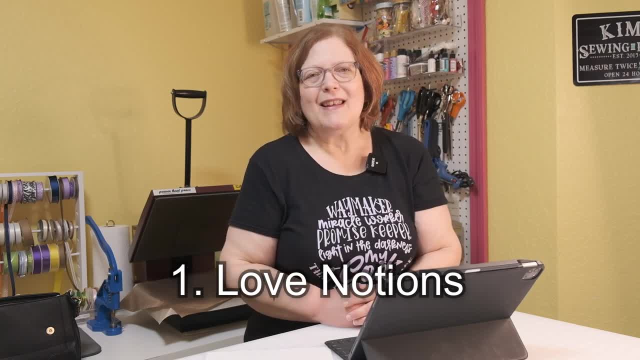 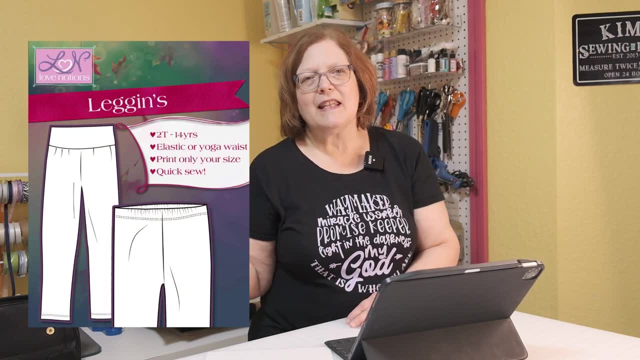 Love Notions. They have three free patterns for kids. The first one is called Love Notions And the second one that I have actually made. this one is the leggings. They're 2T to 14 and they're just like you know the name implies They're basic leggings, but they fit really well. They. 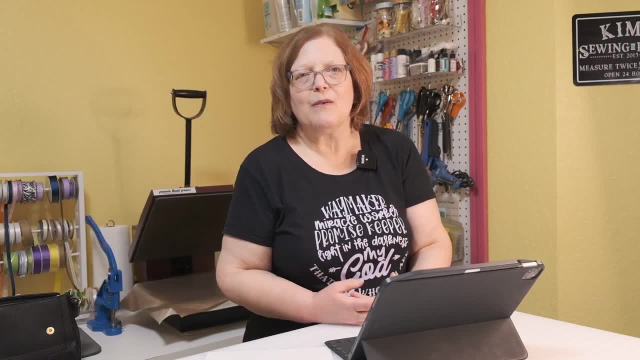 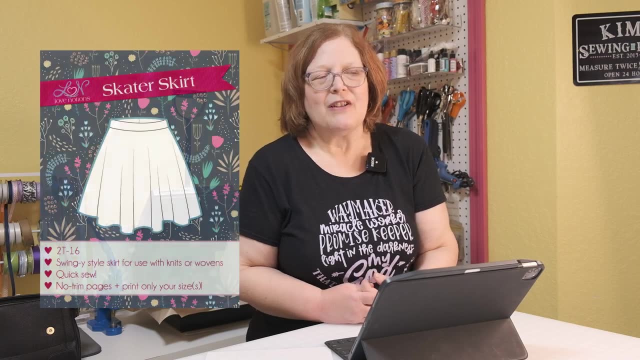 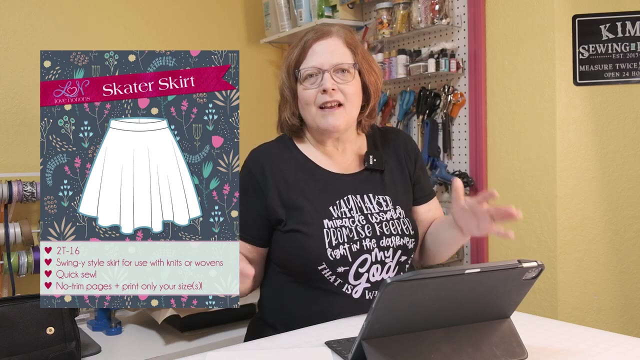 wear. you know, depending on what fabric you use, you can make them to be a really true staple in your child's wardrobe. The other one is a skater skirt, which is just adorable. It's like a swing skirt. I think it might be half circle, if not full, And it is a full-length skirt And it's. 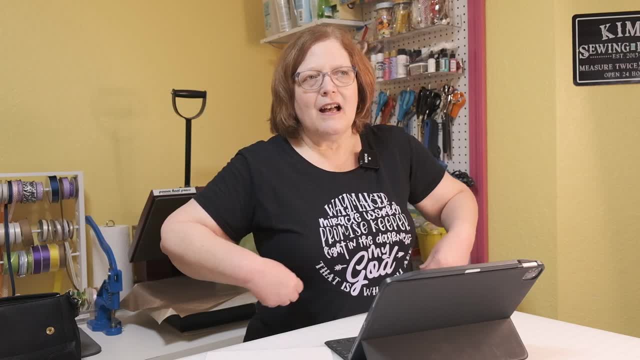 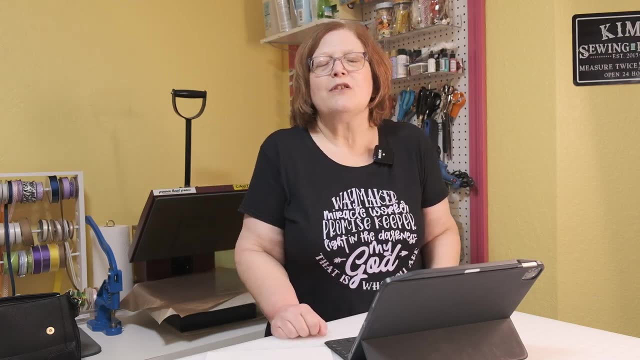 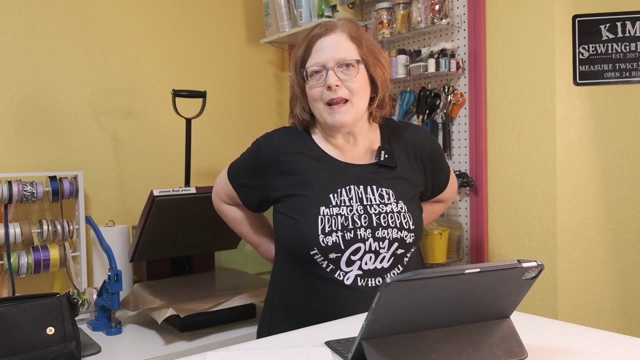 a fantastic little thing that you can actually attach to a waistline and make it into a dress. So you could use any of the tops on Love Notions and do that, Or you could even just use the top of a different from a different designer, as long as you make sure that the waistline's in the right. 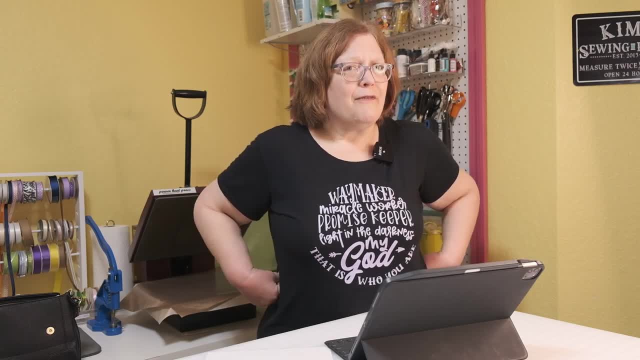 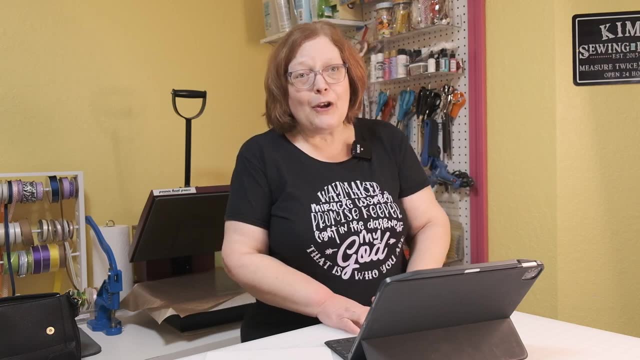 place and that the measurements aren't too far off from each other. With knits it's a little forgiving, So, um, you should be able to do that. The third pattern is the dashing vest, And this is the cutest little thing for little boys. This is the one I haven't made. 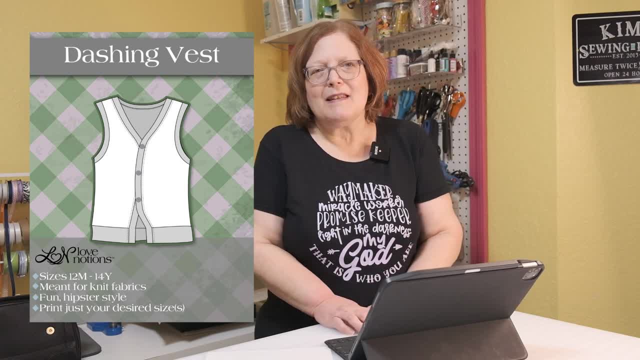 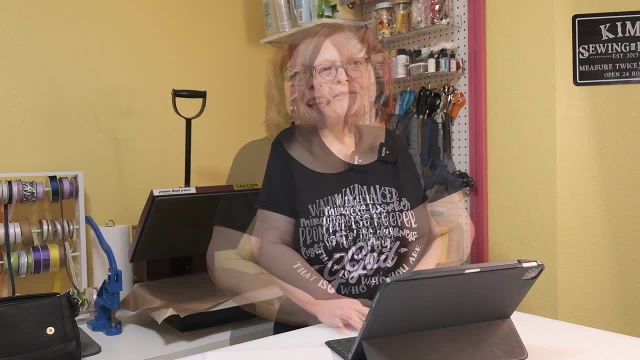 but, oh my goodness, for my little grandsons I definitely want to make this. It's such a little man thing and so cute, And it goes from 2T to 14 as well. The second designer that I'd like to talk. 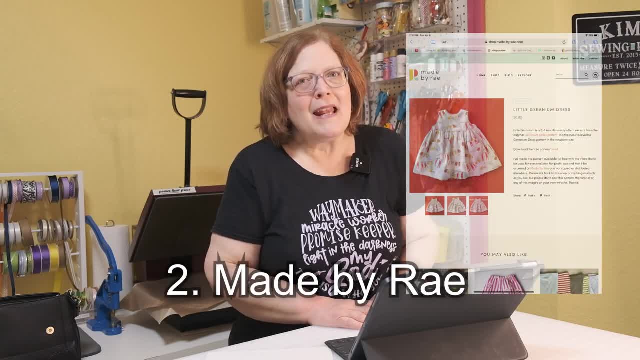 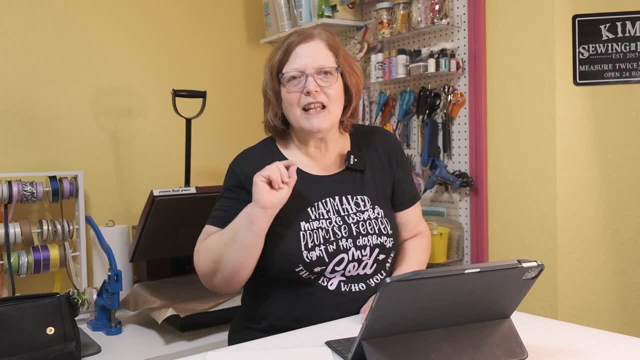 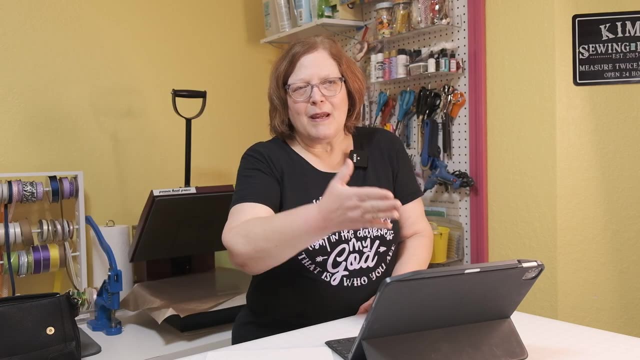 about is made by Ray. As you know, the geranium dress is one of my favorite things for kids And I. that is not free for every size, but they have this little itty bitty it's called, which is basically like a geranium dress And that's for- uh, I think it's three. 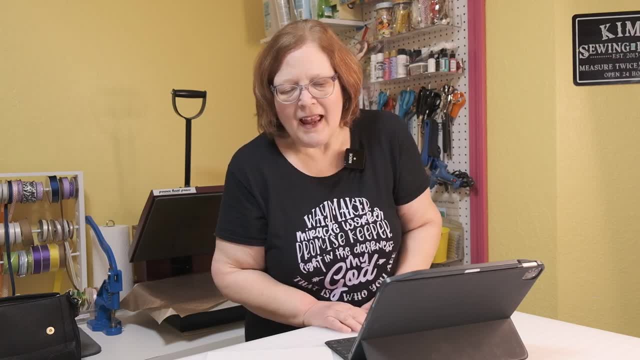 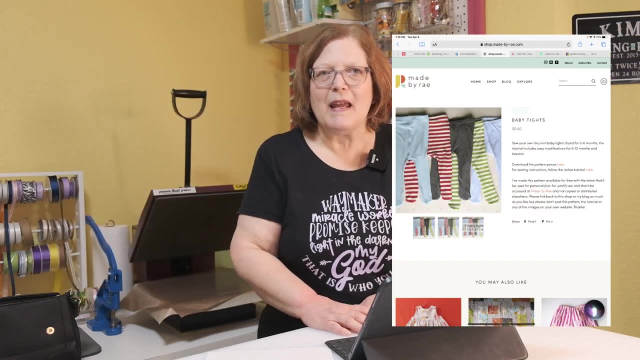 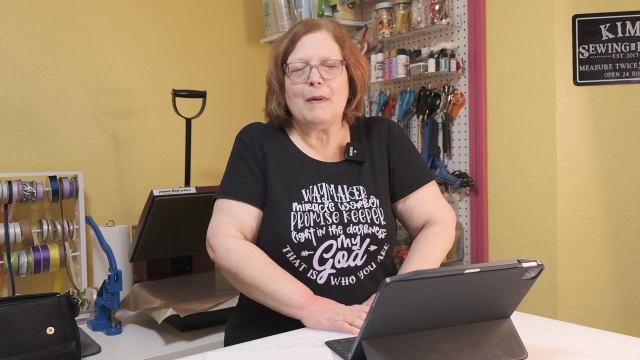 months and younger, but super cute. They also have um a newborn baby pant, which is really handy to have, And they have tights. they have tights for babies. So if the little girls they need tights under their little dresses, you can make them. Um, I think double brush poly is. 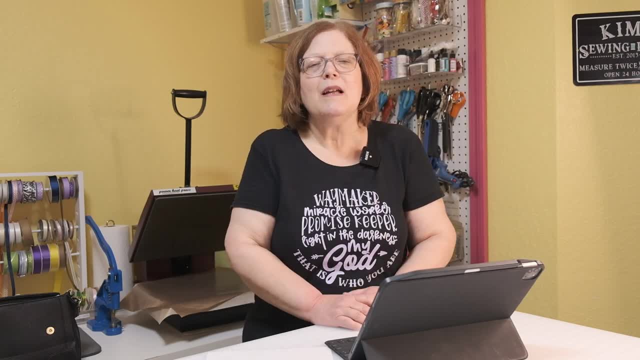 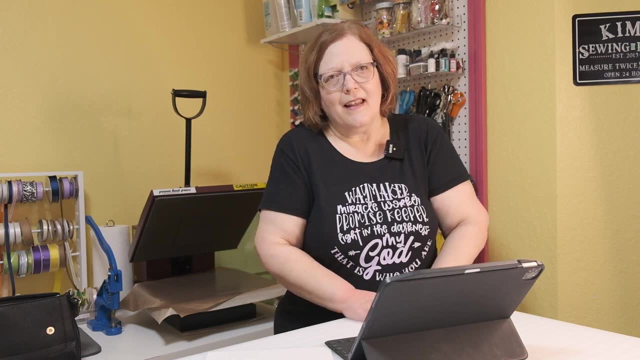 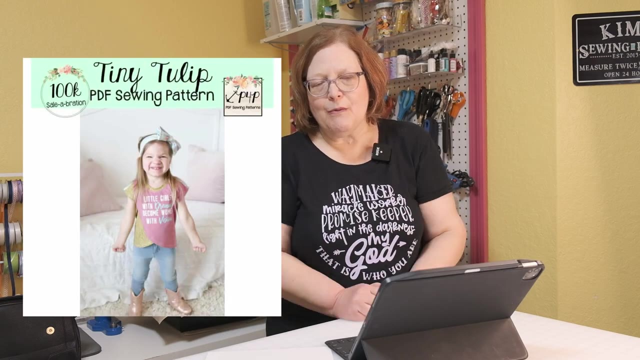 a fantastic fabric to use for that, because it will also be warm. So there's the place you can get your tights for your little girls. So that's made by Ray. The third designer I'd like to talk to you about is patterns for pirates, And they have a lot of free kids patterns. They have a tulip t-shirt. 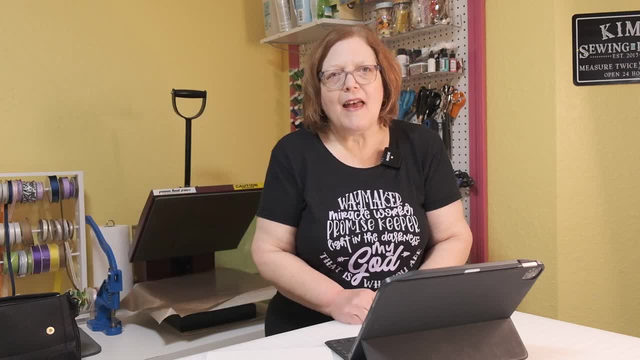 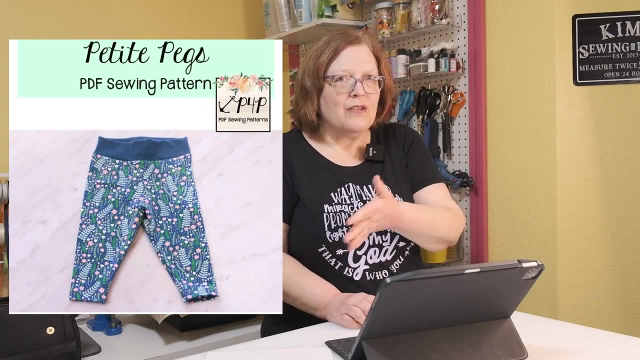 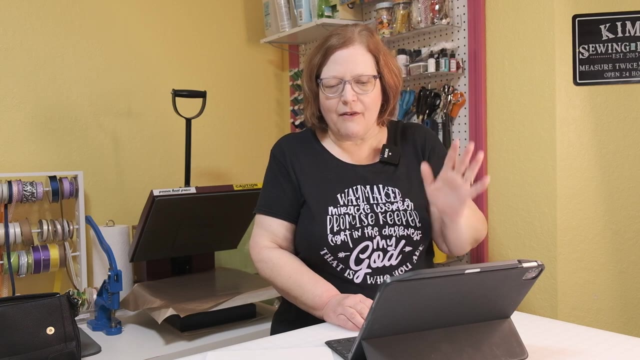 which is super cute for little girls. They also have the wheel at T, which is for babies up to 12 months. It also has um the little pirate pegs, and that goes to that's really all ages. They have them for children, They have them for babies, They also have them for adults and those are free. 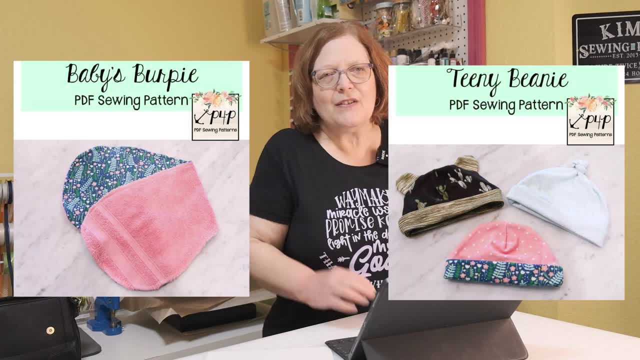 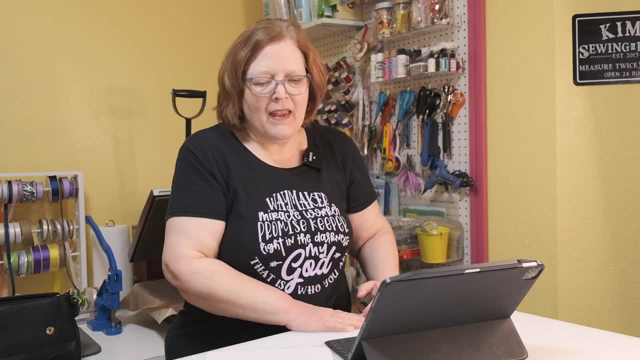 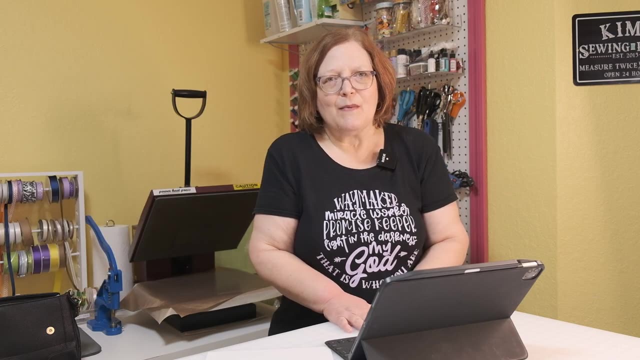 And then they have a burp cloth and a little teeny beanie, which is adorable, And so it's really a whole baby layout that you can make with all of this. And they also have for kids their walk the plank PJ bottoms, which are really, really nice to have. as well, You could go to patterns. 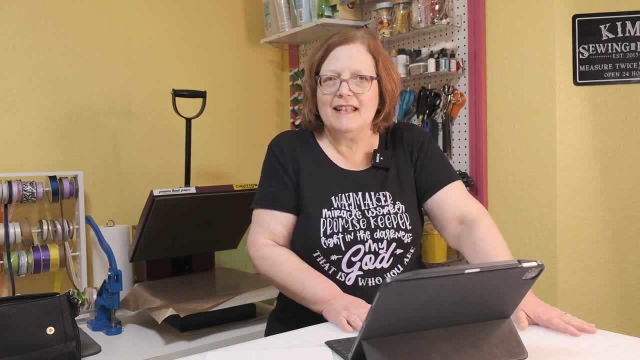 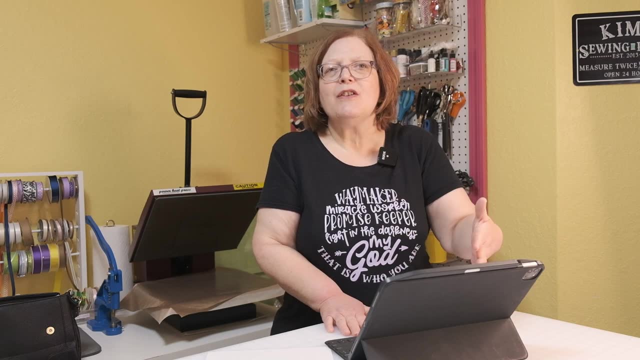 for pirates and make baby gifts from now to keep until the end of time. So just go ahead and check those out. Most of these designers entail, uh, having to join their Facebook groups, So go ahead and do that If they require you to. 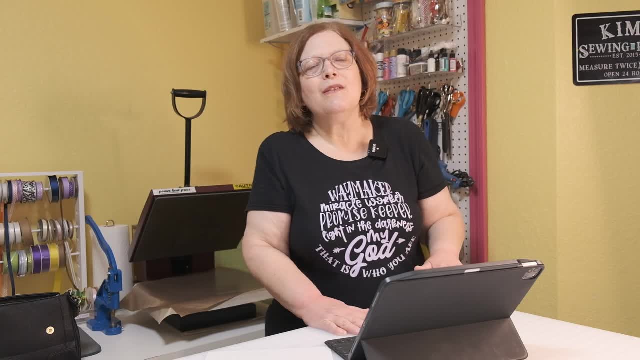 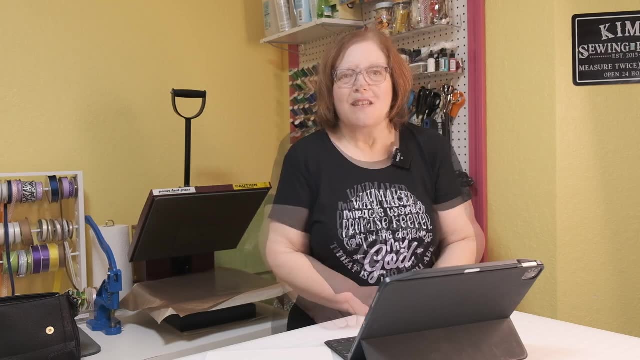 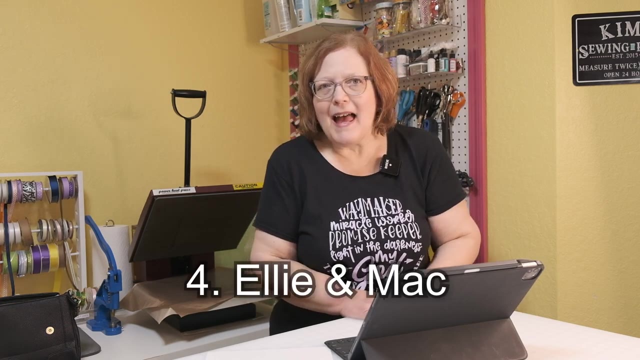 they might not look free at first until you go ahead and do that, And then they'll show up as free, But I think those are free even if you don't, So definitely a win-win there. So the next designer that I like this will be number four for, uh, free patterns for kids- is Allie and Mac. 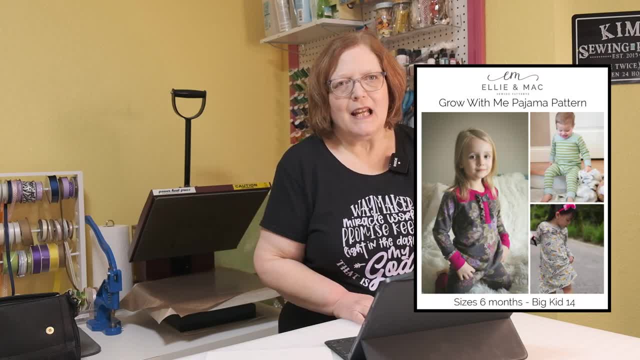 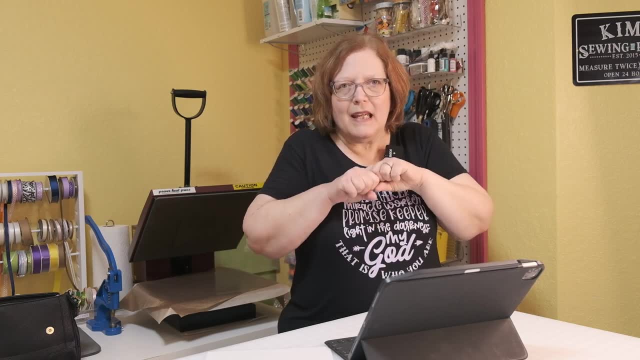 And they have the grow with me jammies, which these are really really nice to make because they have long cuffs And they have a little bit of a uh, a little bit of a uh, a little bit of a on them, on the legs, and you can turn them up in the beginning and kind of let them out as they. 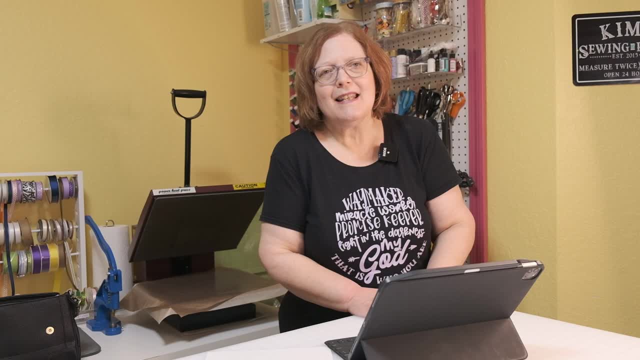 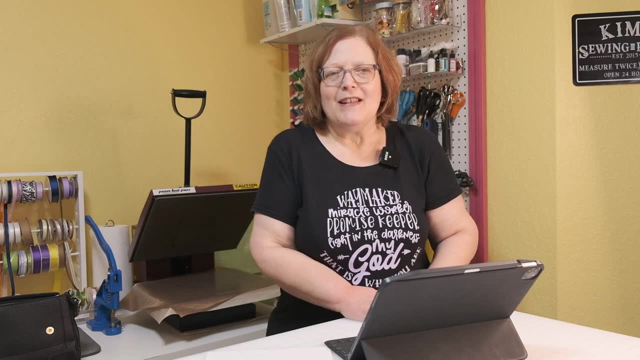 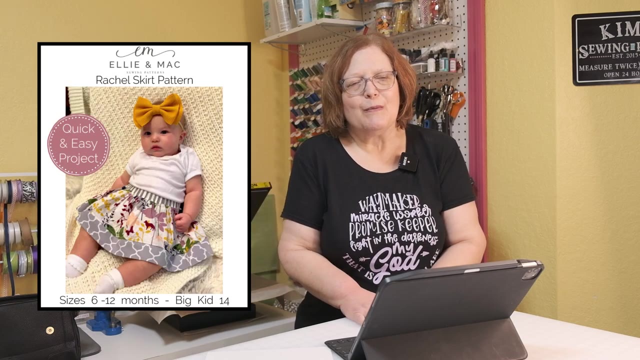 grow, So they really last them a long time. I sent some to my nephew's little boy and he wore them for like two and a half years, So it's a great way to give a gift that will last a while. They also have a little skirt for baby girls, which is really really cute as well. 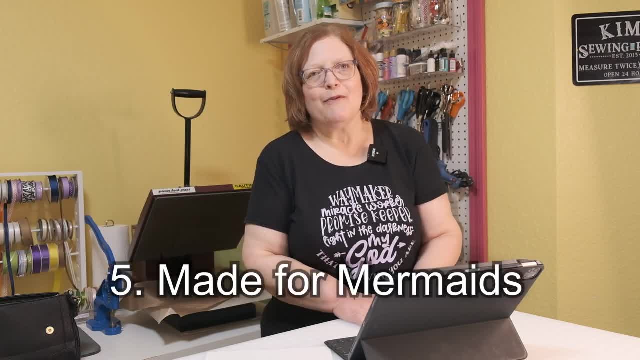 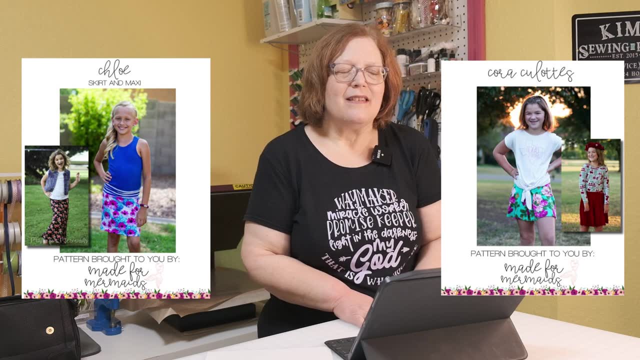 All for free. Number five designer is made for mermaids. Made for mermaids has the core culottes and the Chloe skirt for little girls, And just I mean, they're just beautiful. They're staples and made for mermaids. patterns are wonderful. 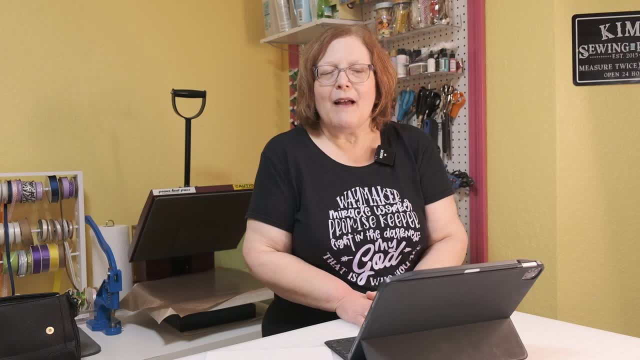 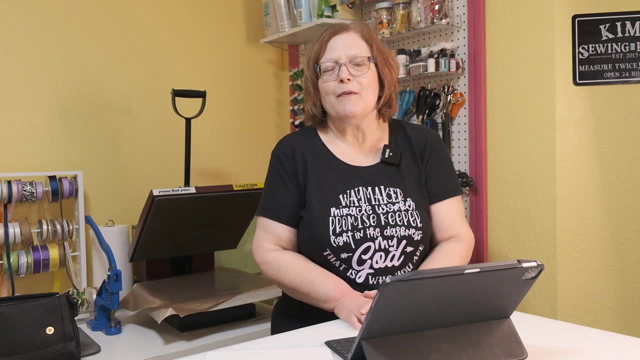 They have great directions. A lot of them have photographs for the directions, which I really appreciate, Uh, so definitely try them out, And I do believe you have to be a member of their Facebook group to make that free. The next one I've already reviewed for women, um a free pattern. 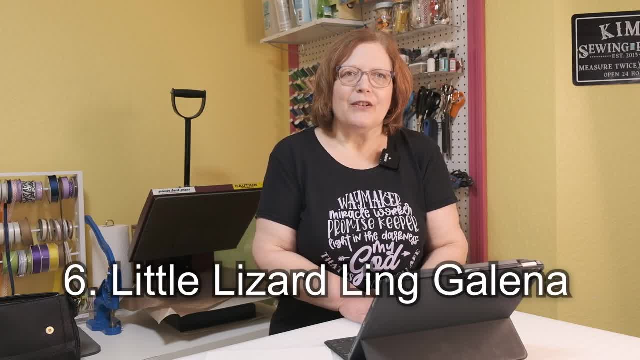 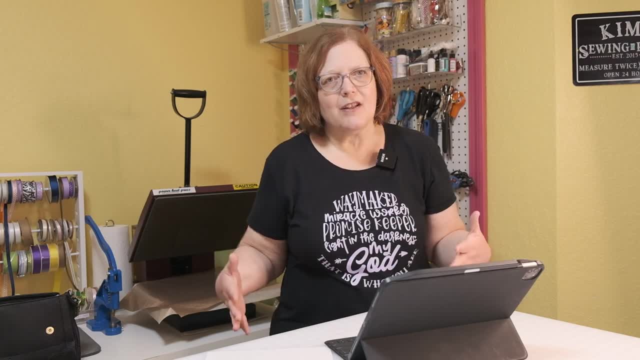 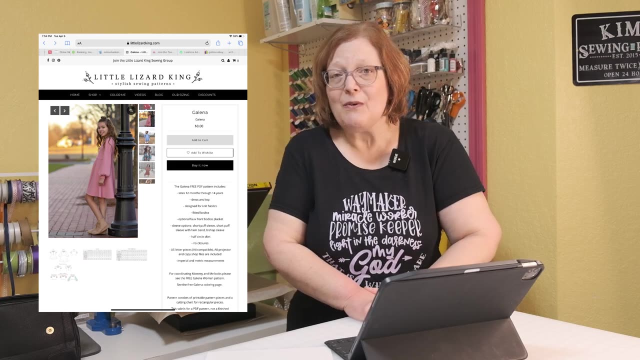 is the Galena from little lizard King. Little lizard King is my hands down favorite kids designer. They have beautiful dresses- I mean drop dead gorgeous, And the photography on that site is beyond amazing. So their free Galena pattern is also available for kids, And Galena is just a. 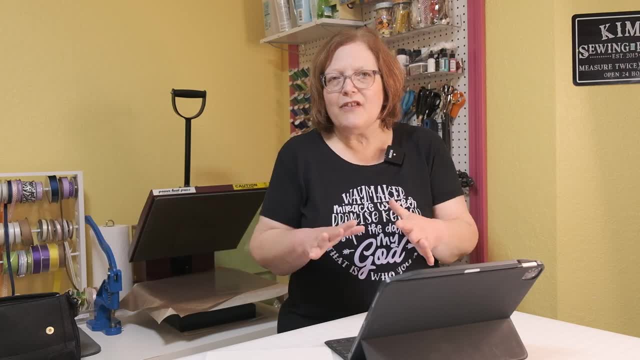 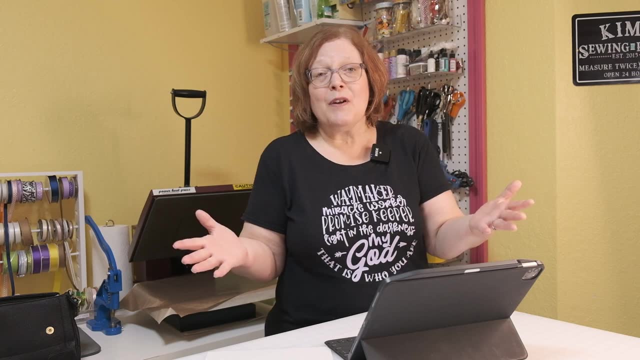 nice little swing dress. Um, like a fit and flare, super cute. Um, doesn't take much fabric for kids And uh it, it's a wonderful gift. I haven't made it for kids, but I've made it for me and I love it. 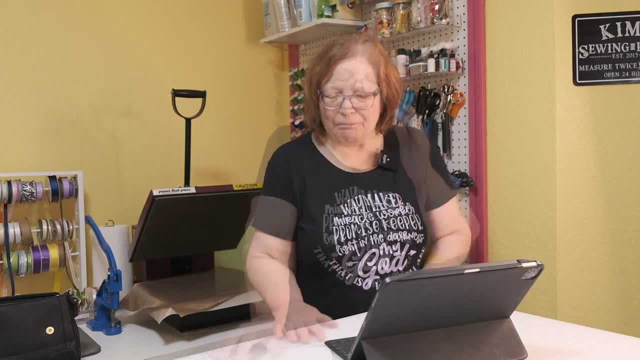 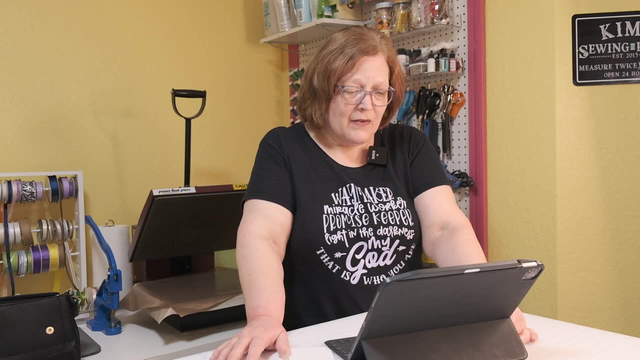 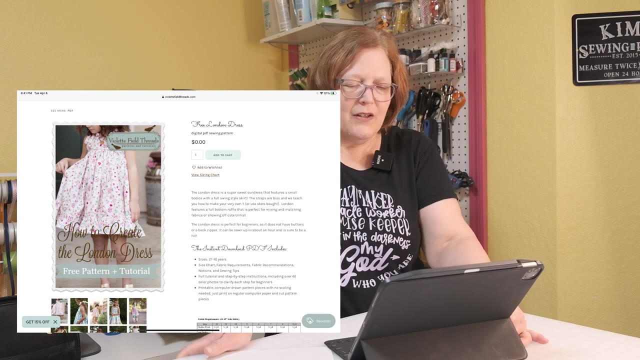 So definitely, you don't want to miss that one. The next one is violet fields threads, and they have a lot of kids patterns that are free. but just to highlight a few, they have the London dress for girls. It's like a pillowcase dress, really adorable, with little ties on those shoulders. 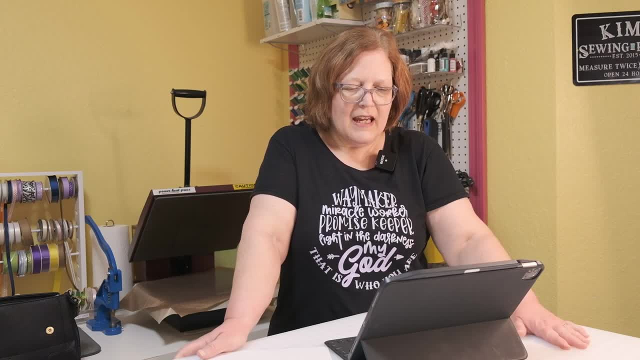 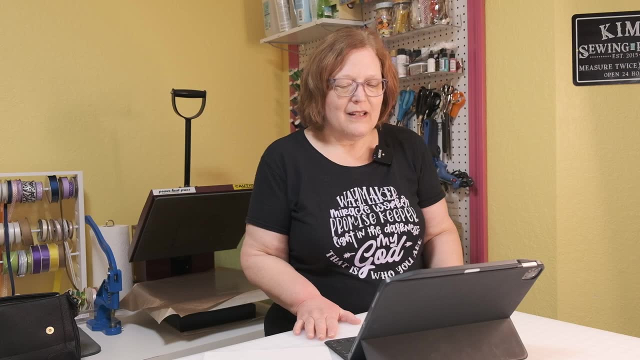 And the other one that I think is really, really useful are the shorties and their little ruffled pants that you can put underneath dresses or tops or whatever you like. really cute, Um, so definitely. they have a lot of doll things too on there. So, um, if you 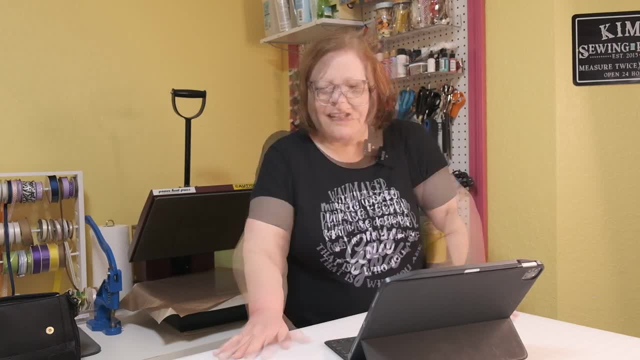 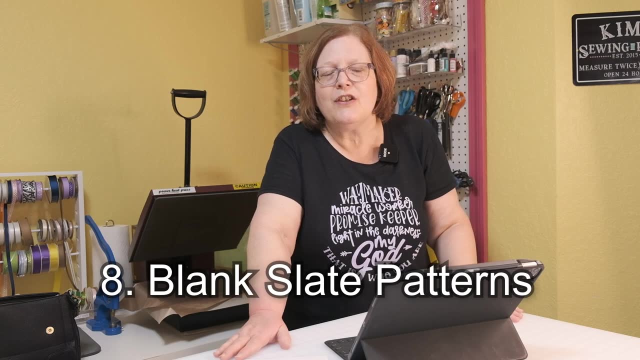 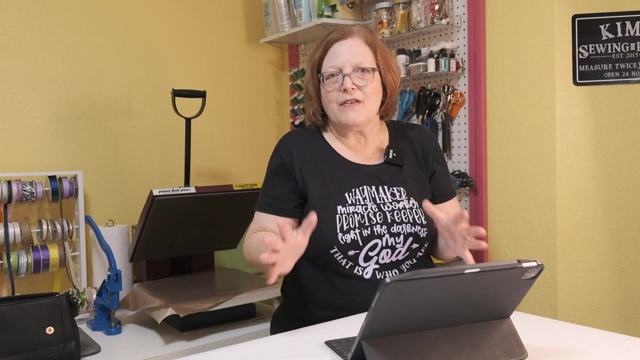 have little girls. you definitely want to check that site out. Number eight is, uh, from Melissa Mora at Melly's sews and she has blank slate patterns and she has a little boy's t-shirt. She also has a little pinafore for babies and little um diaper covers. 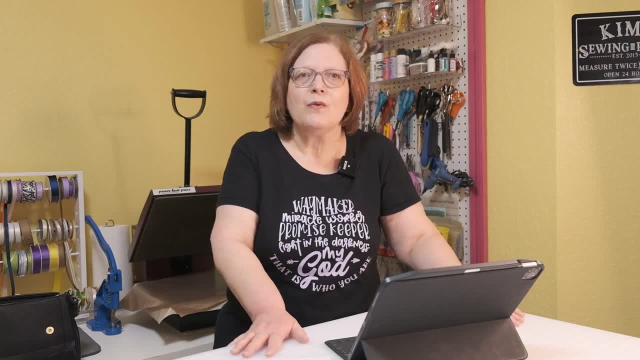 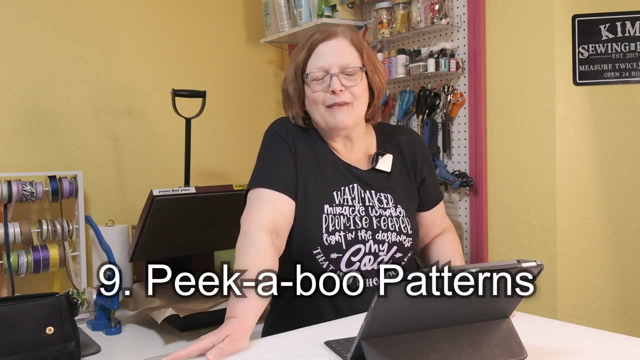 So really cute. I do think you have to join her newsletter in order to get the free patterns. Number nine is peekaboo patterns, and they have very, very adorable things as well. They have a few things for adults, but they're mostly kid designer. 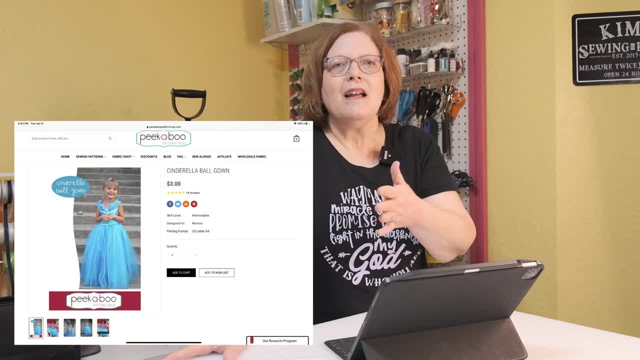 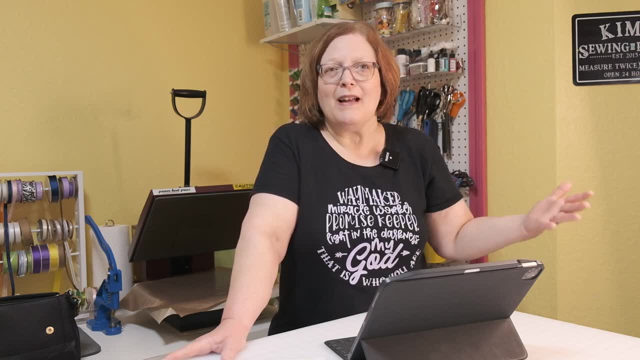 They have a Cinderella dress which is actually a replica in the new Disney Cinderella. Just adorable, I haven't made that. I I've made that pattern, but not, uh, theirs. I've made that Cinderella dress. Um, I think it's really, really cute. And then the next one is: uh, 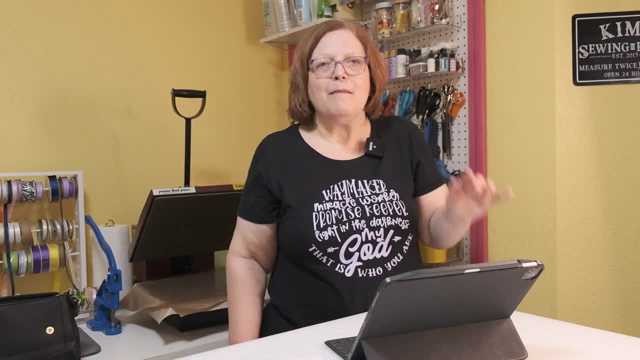 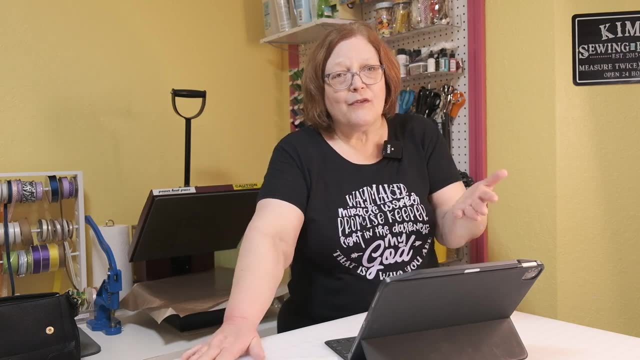 I think there was a simplicity one out right when the movie came out and I made it for um. I made the doll version and I also made the little girl version, but they have a dress on there and it's free, And they also have um PJ party pants that you can make pajama. 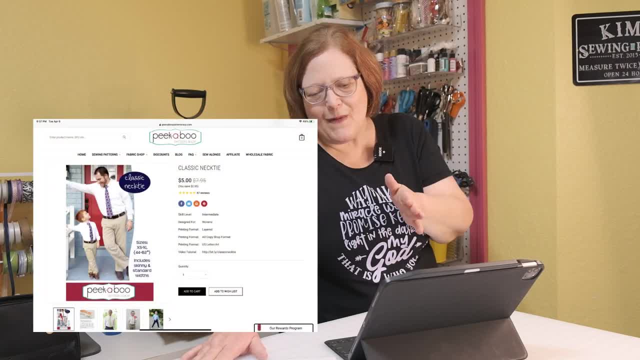 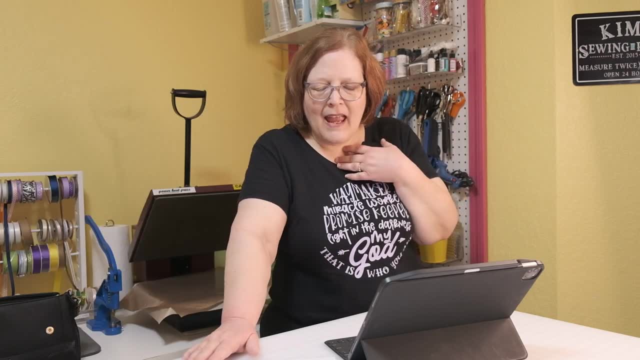 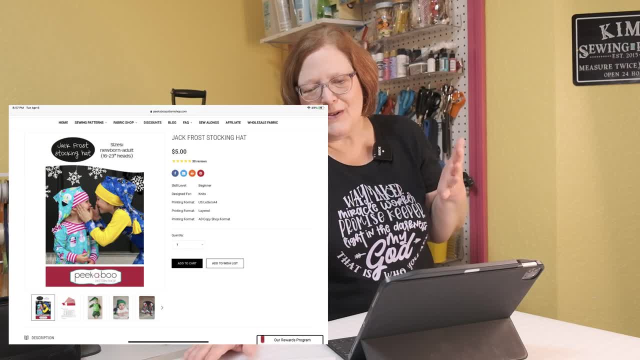 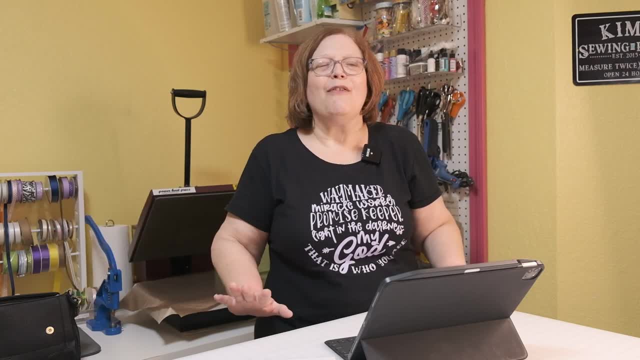 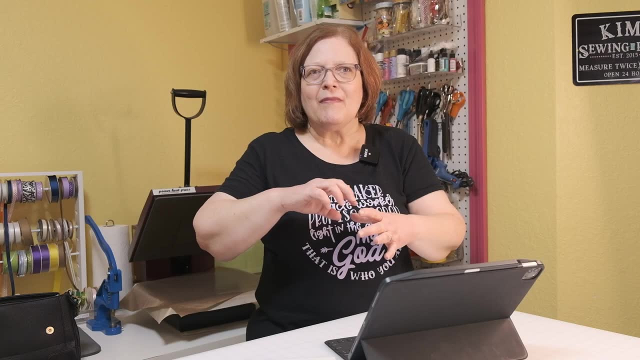 And they also have. you guys, This is the best idea ever. They have this little thing called the tinkle TP, And what you do is you actually? um, they're just like a little cone shaped thing that you actually put over the little baby boy while you're changing. 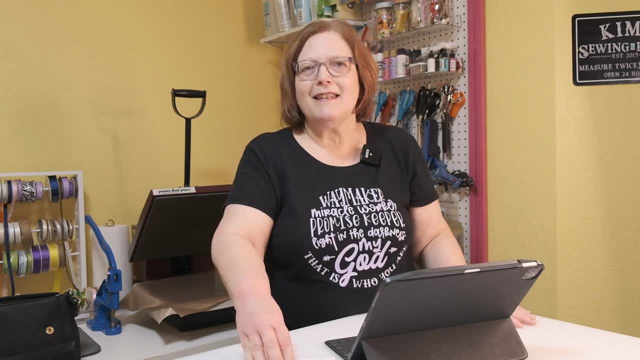 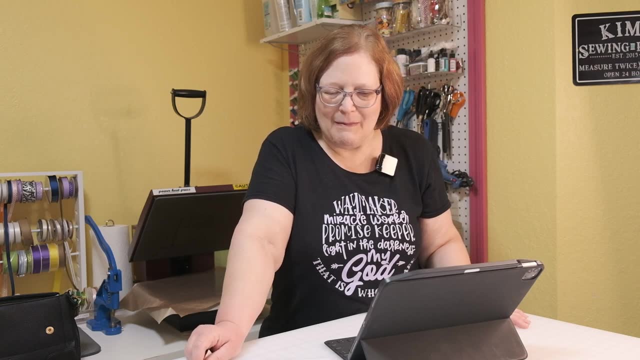 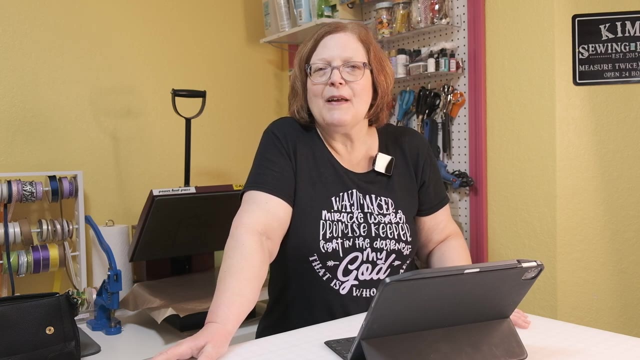 a diaper to keep from being in debt. Okay, Really, really cute, great baby shower gift. I think that new parents might find it really amusing and I really really enjoy those patterns. I have made some of those, but not all of them. 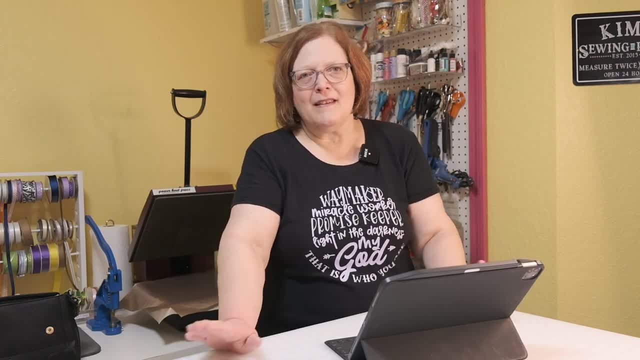 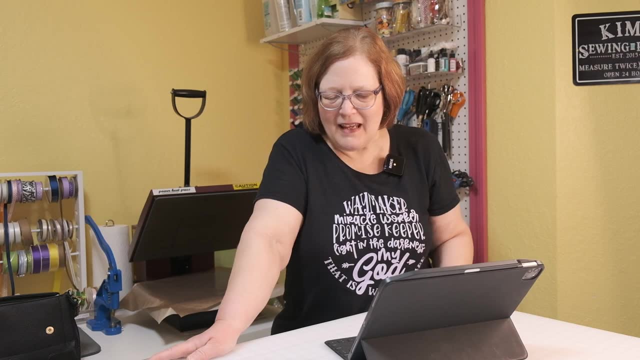 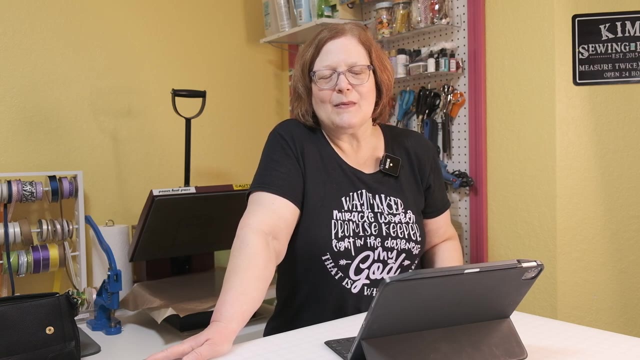 So, anyway, that is adorable and I downloaded that because the very next boy baby shower that I go to is definitely that's gonna be included there somewhere. Also, number 10, and this one is Sew a Little Seam and she has some adorable patterns for kids as well. 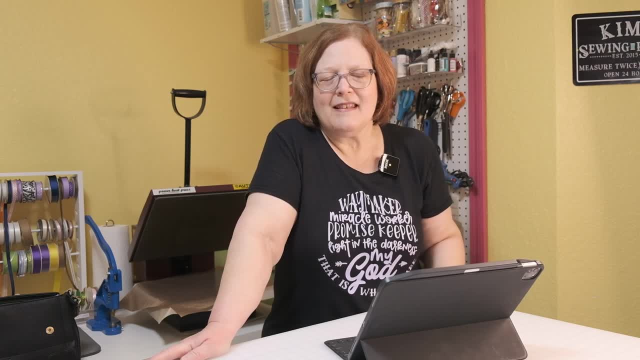 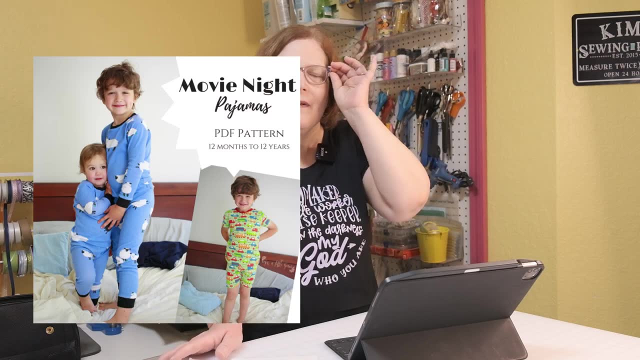 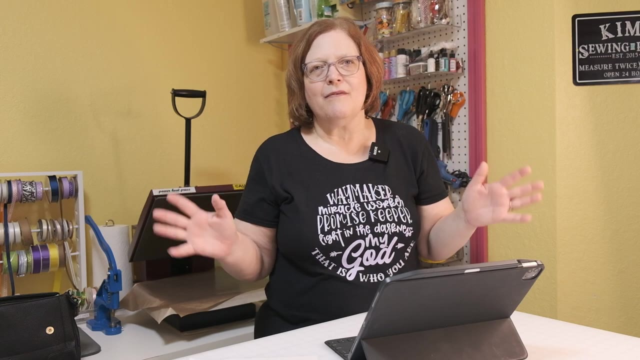 She has some pajamas also and I have made these. I made many pairs of these and it is the movie night pajamas and they have a couple different options of sleeves and you can do a Henley type top and just a lot of variety that you can do with it. 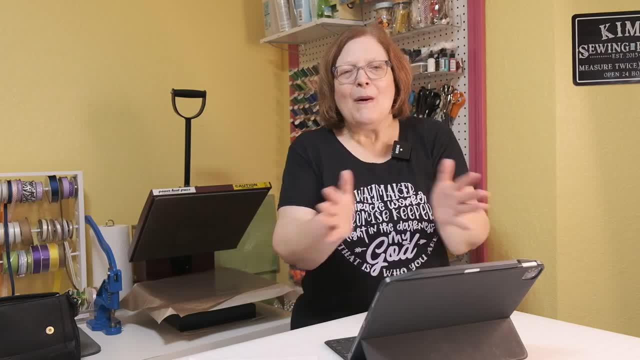 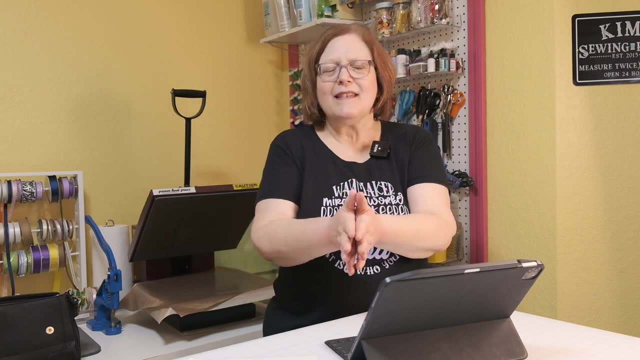 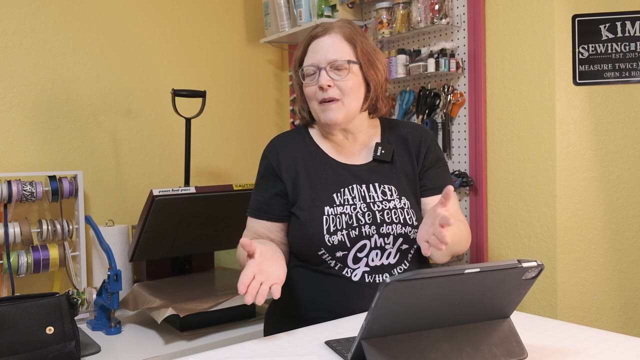 and they are free, So I hope that gives you a start in sewing for your kids this spring and beyond. Most of these PJs can be made into shorts too, so you can have summer PJs or winter PJs. You know kids need warm things all year round. 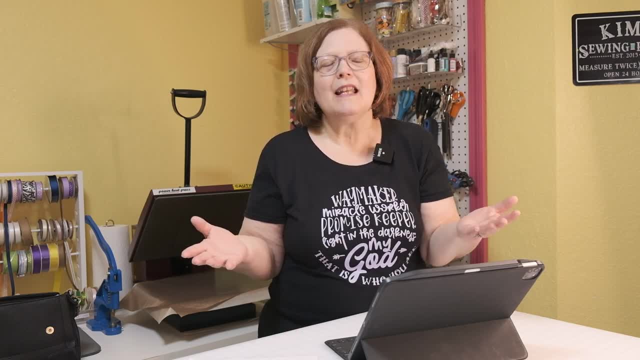 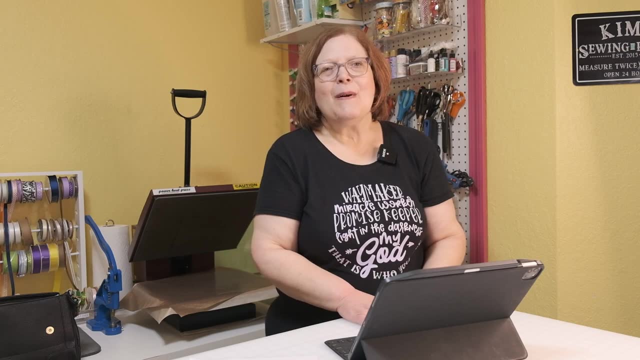 no matter where you live, It gets sometimes a little chilly at night everywhere, So definitely you're gonna wanna stock up on those things for your kids. So I want you to have a great day. I hope all your sewing adventures are successful. Have a great day. 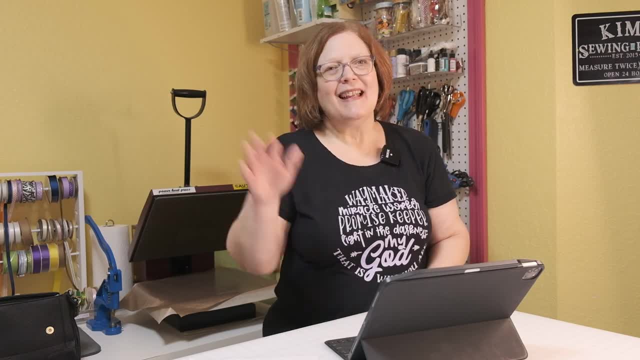 Be successful this week and I'll see you in the next video. Happy sewing.